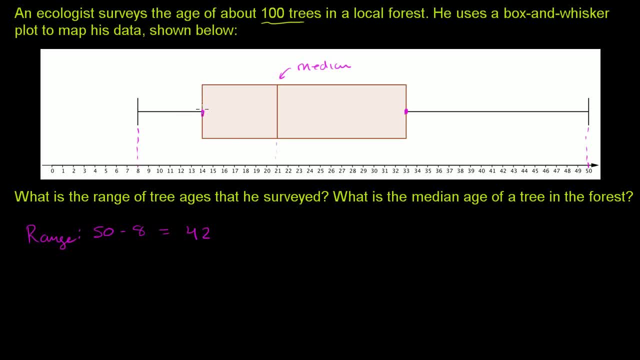 or older than 21.. And so these, essentially, are splitting. We're actually splitting all of the data into four groups. This we would call the first quartile. So I'll call it q1 for a first quartile. Maybe I'll do one q. 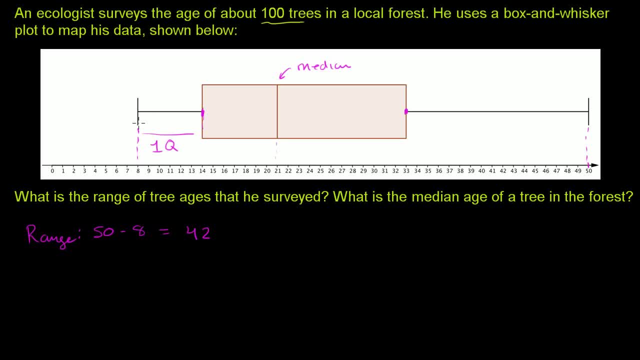 This is the first quartile, Roughly a fourth of the trees, because the way you calculate it, sometimes a tree ends up in one point or another. about a fourth of the trees end up here. A fourth of the trees are between 14 and 21.. 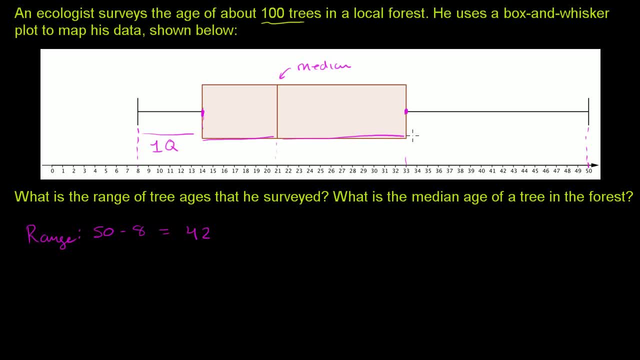 A fourth are between 21 and it looks like 33.. And then a fourth are in this quartile. So we call this the first quartile, the second quartile, the third quartile and the fourth quartile. So to answer the question, we already did the range. 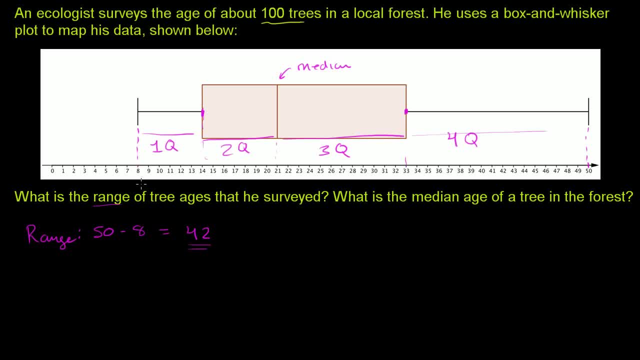 There's a 42-year spread between the oldest and the youngest tree, And then the median age of a tree in the forest is at 21.. So, even though you might have trees that are as old as 50, the median of the forest is actually. 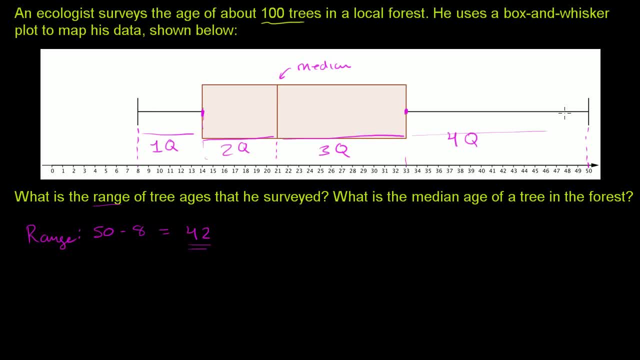 closer to the lower end of the forest, The lower end of our entire spectrum of all of the ages. So if you view median as your central tendency measurement, it's only at 21 years And you can even see it. It's closer to the left of the box. 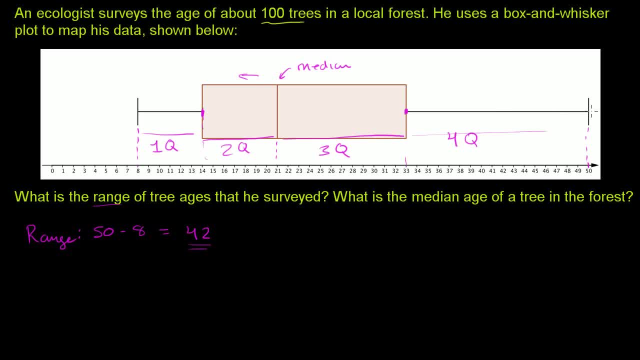 and closer to the end of the left whisker than the end of the right whisker.